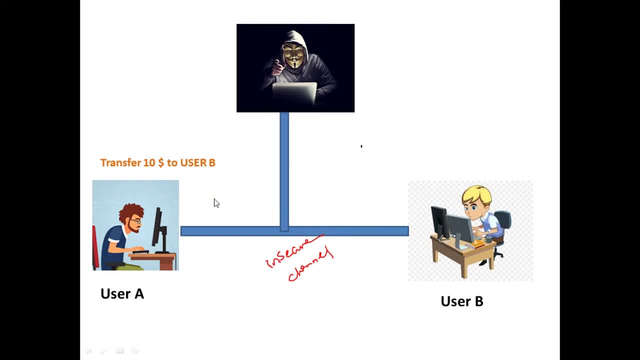 Say he's transferring $10 to User B to user b, there's always a chance that this communication can be captured by your hacker and he can say: convert it to thousand dollars and send it to user b. so the transfer of ten dollars has now been changed to thousand dollars, say, from user race account, instead of ten dollars thousand. 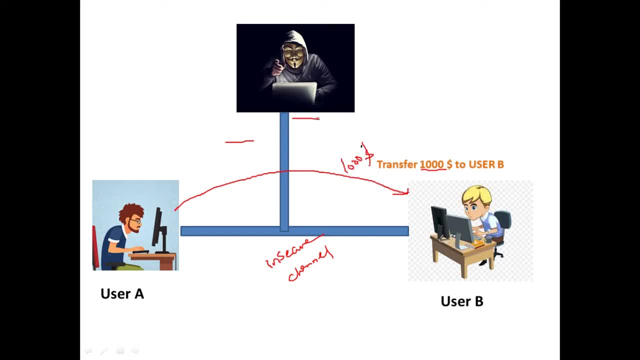 dollars got transferred because the message was altered by this particular hacker. so in that case, you'll know what will happen next. that is, uh, what we can see. let's consider is user a and he is user b. this is going to be the scenario, because when a thousand dollars get transferred instead of a ten, 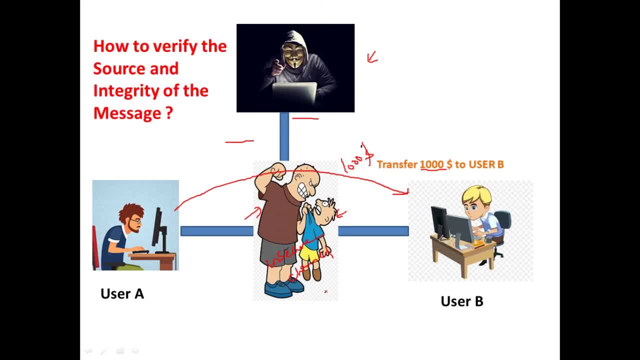 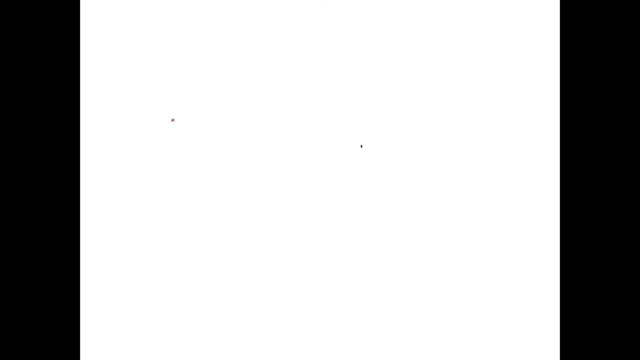 dollars, we're going to have some issues. so now, how to verify the source and integrity of the message is the question. we'll now take a look at the solution to this problem using digital signatures at a higher level. again, we have this user a and we have 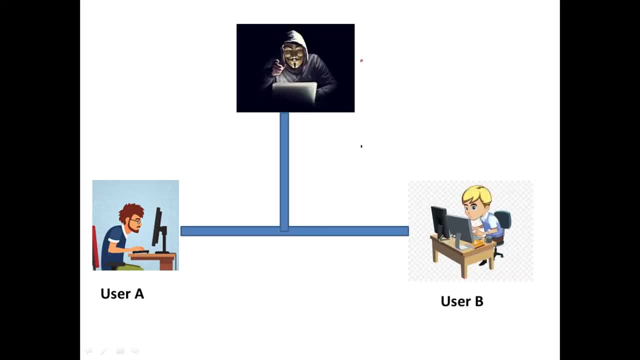 user b. they are communicating over this insecure channel, so, as usual, we have our hacker. the very first step is: user a generates a public key and he has also a private key, so two keys for this user and this public key is shared with everyone. it's public, so everyone knows the public. 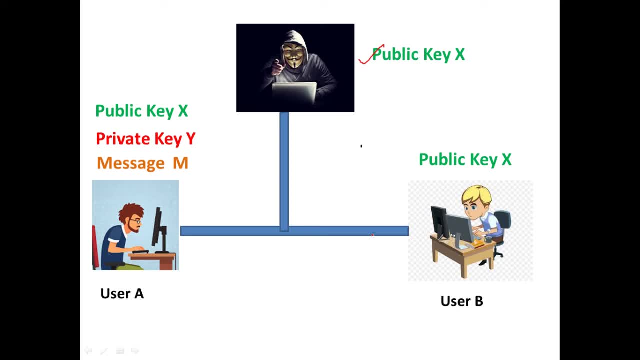 key of this user a and whenever user a wants to send a message, what he does is he takes the private key and the message and then he converts that to a signature. say, let's assume that this is the signature r comma s: after creating the signature, using the private key, is going to attach that with the plain text. 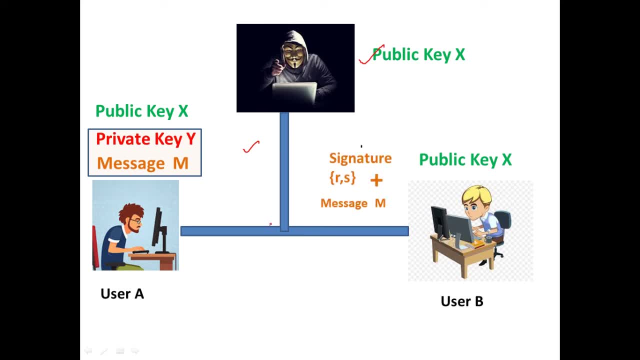 message and is going to send the signature along with the message to user b. so what user b can verify is he can use the public key. so he can use the public key and he can verify whether the signature is valid or not. so we can verify two things: we can verify the integrity of the message. we can also verify the.